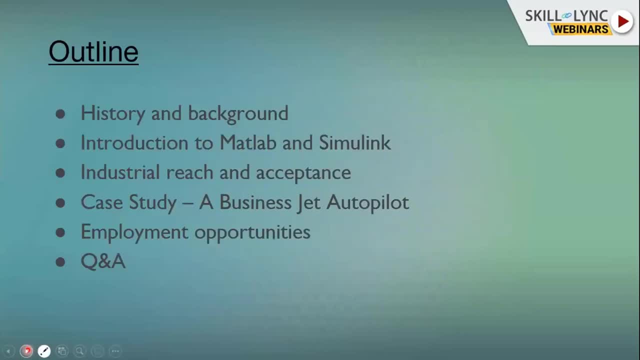 That is, the aerospace industry. So the outline for today's webinar is: I'm going to dwell on the tool set. you know a little bit of history and background on where we started and where we are today in the last 20 plus years And how MATLAB and Simulink tool chain. 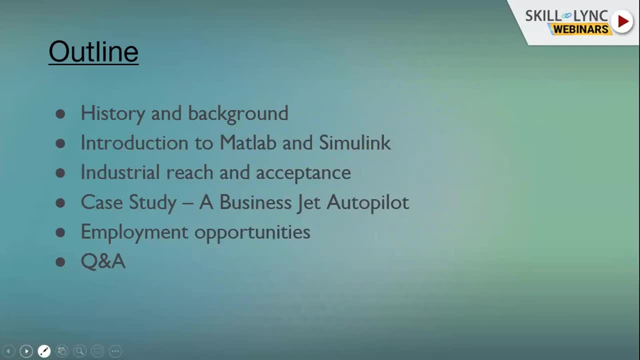 gained the popularity, Followed by: Yeah, an aircraft example. you know modeling an aircraft in a few slides. It may be overwhelming, but please bear with me. I'll try to declutter the modeling aspect And then the case study. 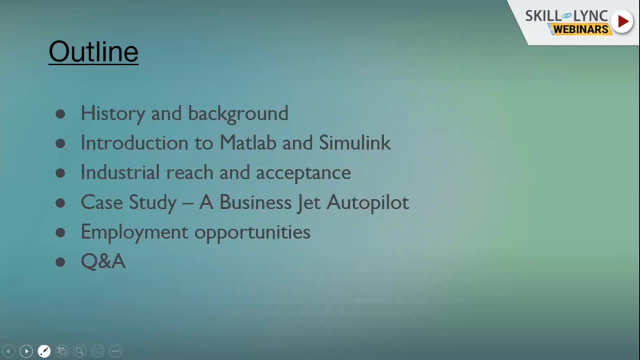 also includes a design, autopilot design, what it would take to design an autopilot using MATLAB Simulink toolchain, And I'm also going to touch upon what one could expect with the MATLAB Simulink training. you know, because I take it you know all participants. 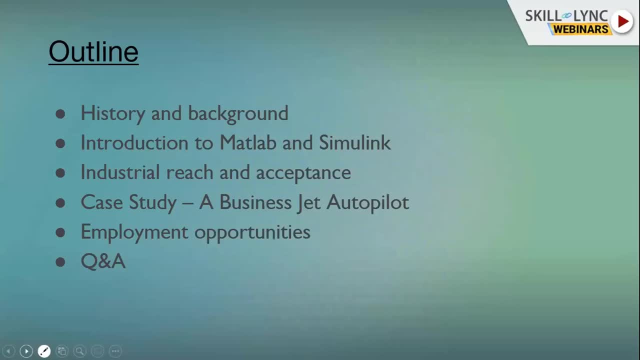 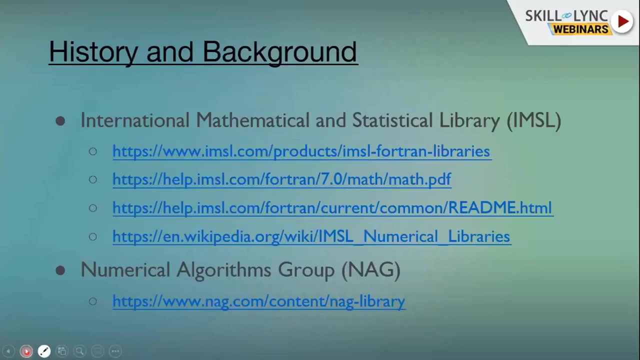 are engineering students, you know, in related areas, trying to learn about MATLAB and Simulink and see how it can be used. So I would conclude with employment opportunities, followed by a quick Q&A. So a little bit history and background on the tools. Like I said, I've been in this area for a good 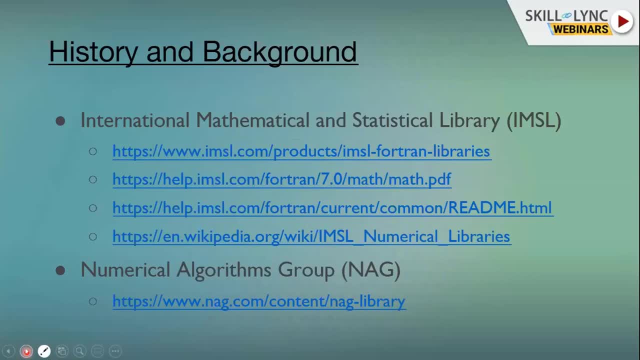 20 plus years And as I was kind of climbing my ladder- you know I was in this area for my career ladder- I was exposed to a lot of libraries. you know they were all in Fortran. I'm going to touch upon those, but I just wanted to list what tools- computational tools- 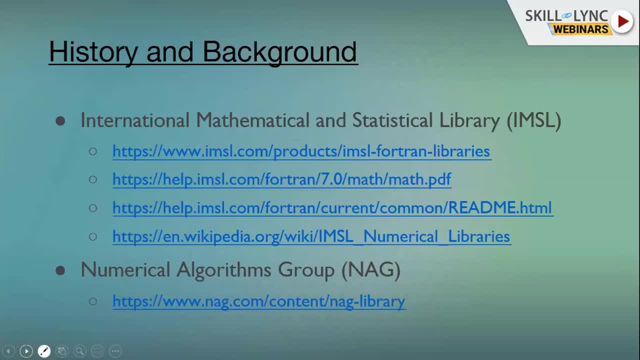 were available to us, you know, 20, 30 years ago. So the IMSL. IMSL stands for International Mathematical and Statistical Library, you know, mainly for statistical analysis. The entire package, Most of these tools, were originally funded. I have provided links for you know interested. 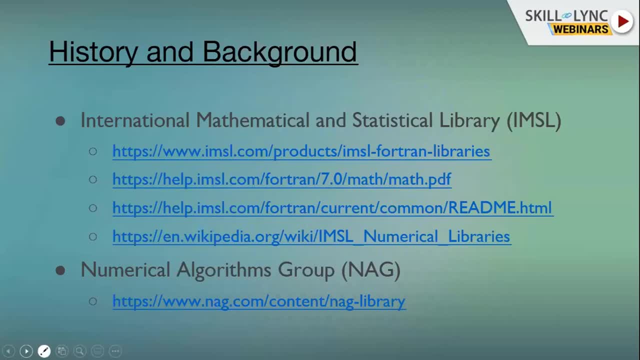 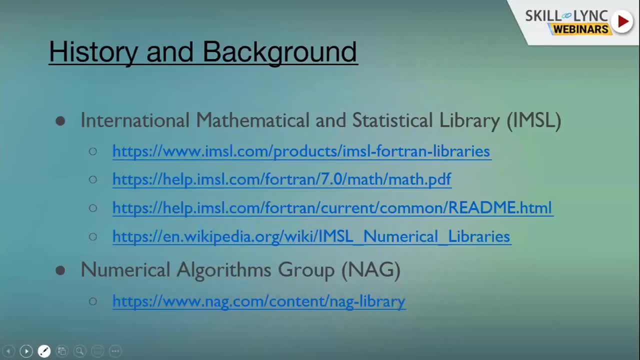 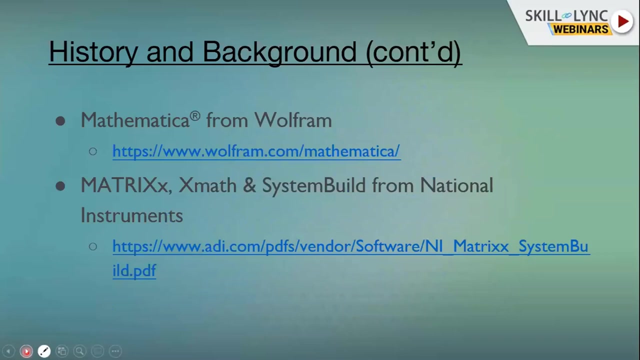 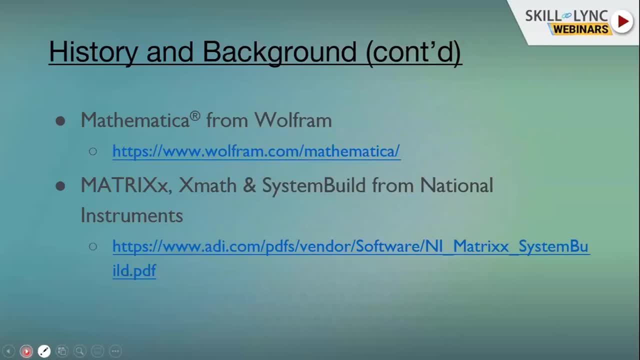 routines who are, were basically for numerical implementations of models or analysis. What Wolfram did was they were trying to come up with a product where everything could be done symbolically so you don't have to keep repeating those computations or derivations and then, when you have a set of parameters, you could quickly turn them on those parameters. 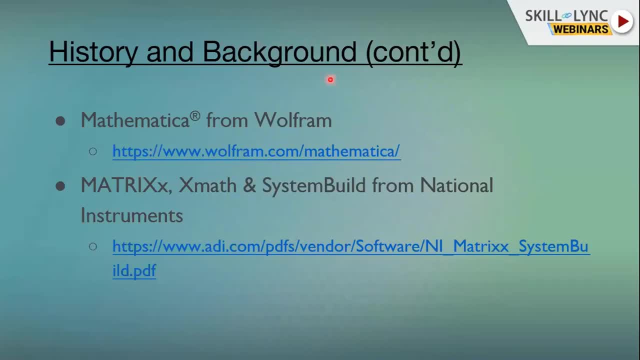 to find solutions. So then there was another contemporary product which was looking more like MATLAB simulink at the time, called Matrix-X. Matrix-X had an xMath component, which was a model that was called matrix-x. Matrix-x had an xMath component, which was: 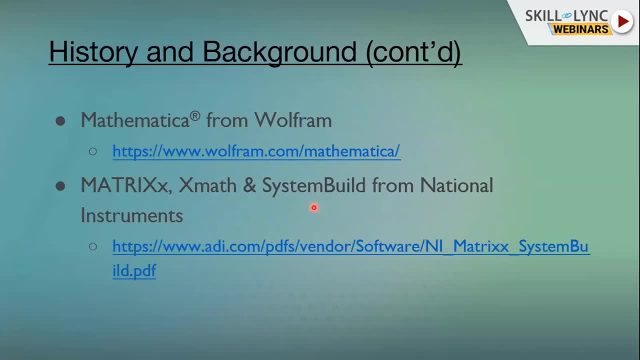 looking more like MATLAB simulink at the time called matrix-x. Matrix-x had an xMath component which was a scripting language support, and the system build is today's simulink from MathWorks And the Matrix-X product again, I think in next few slides I'm going to go over some additional details. 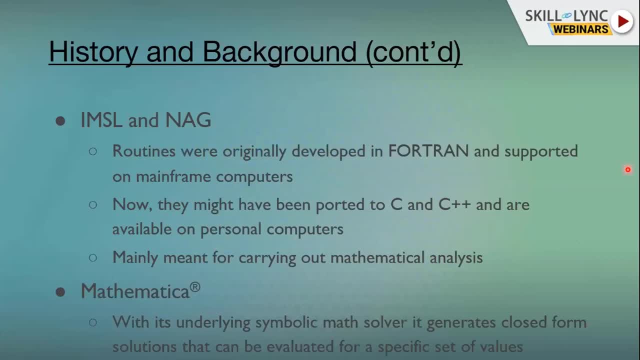 So a little bit on IMSL and NAG. The routines were originally developed in Fortran and supported on mainframe. like I said before, I'm sure they have evolved and now they put in C and C++ and also make them available on multiple platforms like PCs. They were originally developed targeting mainframes. 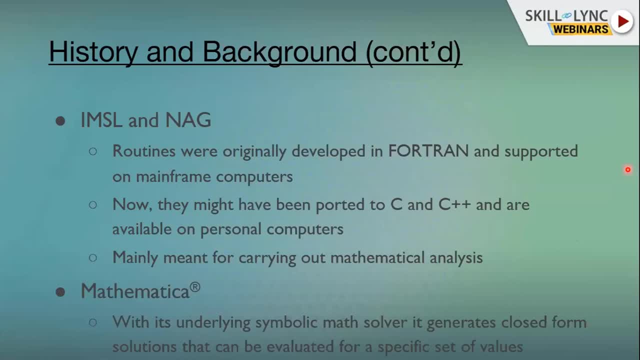 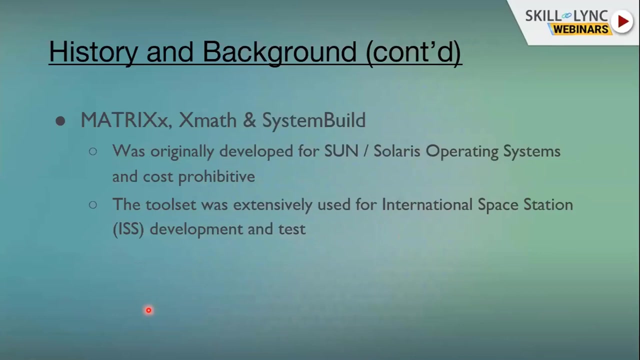 but now to compete in the market they have to put them to different platforms. Mathematica, like I said it had. it still has symbolic math solver. again, you can come up with solutions for specific cases. Matrix-X- I just wanted to share this Matrix-X story. Matrix-X xMath system: build like I said, it was similar to MATLAB and simulink. 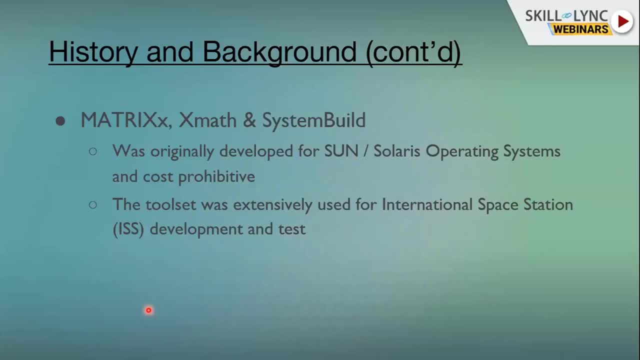 Originally the product was developed for Solaris and Sun operating systems and on expense, But I think, stellen, I know that many of you are aware that the modern space station designed it to be an international space station, because they had not really studied any of the documents and high performance hardware platforms. 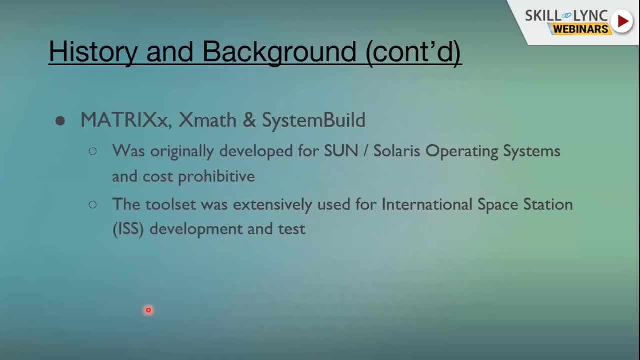 Because it was originally funded by International Space Station program. So they didn't really look at marketing the the product, commercializing the product. instead, they just developed it and used it for International Space Station design, development and tests Because they were adequately funded by the program. they didn't see a revenue generation process. 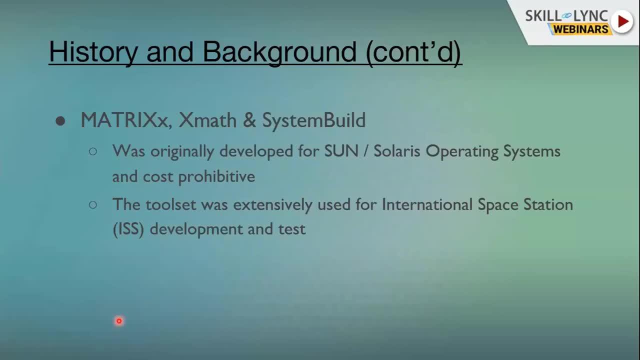 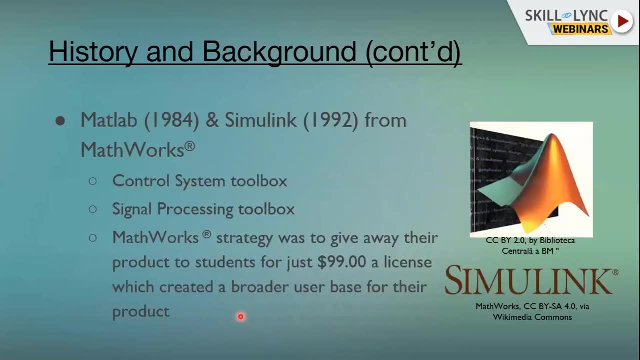 revenue generation process. At least it was not critical for them. And then around the same time even MATLAB and Simulink existed. MATLAB was made into a product in 1984, and then Simulink was added in 1992.. 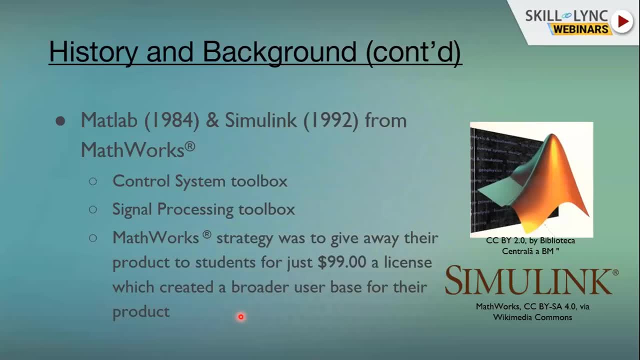 And ever since they were developed and marketed by MathWorks And at the time MATLAB had just two toolboxes: control system toolbox and signal processing toolbox. The researchers and engineers behind MATLAB and Simulink were mainly control system engineers with electrical engineering background and control systems. 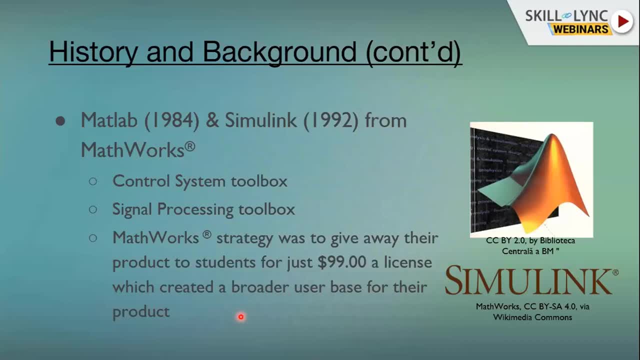 specialization. Signal processing was an add-on. So what MathWorks did was they collaborated with academia, because the academia was always focusing on cutting-edge solutions. So even the control system toolbox would have taken shape originally from an academic institute, And then it was embellished to make it part of MathWorks and MATLAB. 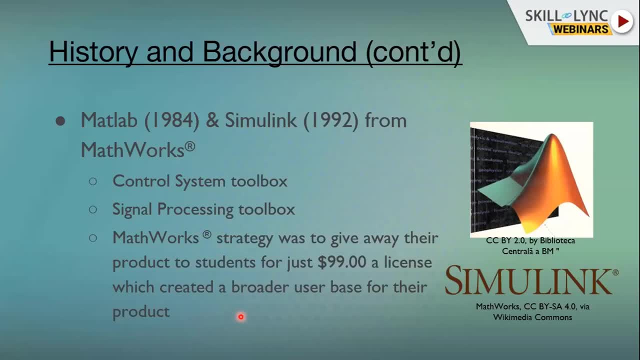 So we have seen how Matrixx- or at least just learned that Matrixx- did not have a strategy to commercialize their product And it was cost prohibitive because it was developed for high-end platforms that used the Unix operating system. The next slide. 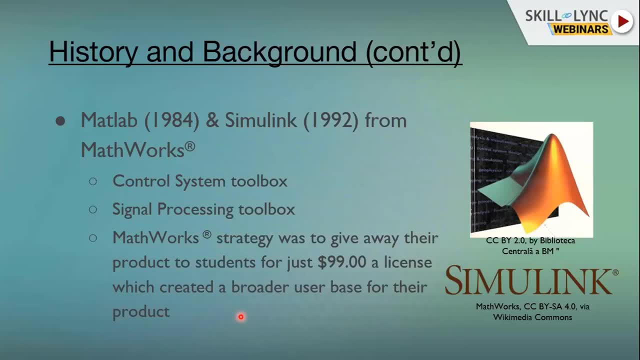 You know now Linux, of course. But MathWorks saw an opportunity And they started giving away their product for $99 apiece, While the Matrixx would have costed someone like $20,000 apiece. So MathWorks, and again. MathWorks did not start from scratch. 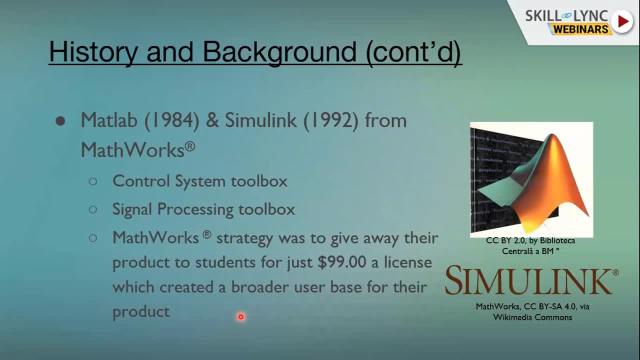 What we have previously seen: the NAG and IMSL libraries. they were basically open-source for most of the engineers and researchers, So they started with the open-source code that was available in Fortran and started building MATLAB. So it was a no-brainer. 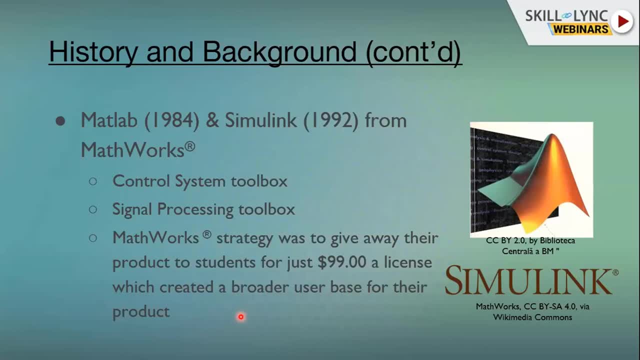 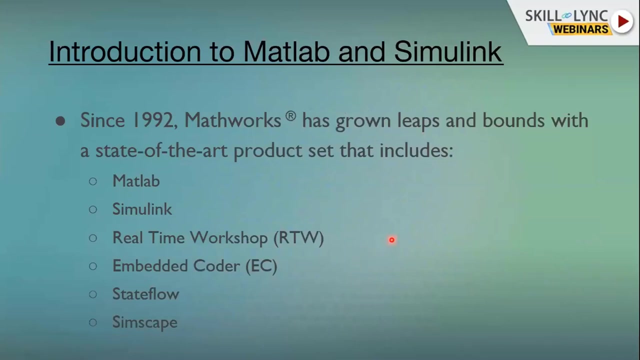 So they tried packaging things and maybe providing additional details how these tools could be used. functions could be used, So it really helped. MathWorks come a long way. So that's essentially a little bit on the history and background. Now let us see where we are with MATLAB today. 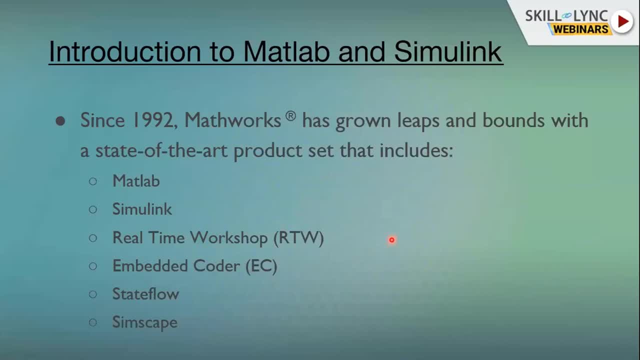 So MATLAB MathWorks has grown leaps and bounds with a state-of-the-art product that includes MATLAB and Simulink. They also have a real-time workshop which helps generating C or C++ code from their Simulink blocks, And then they also have an embedded coder. 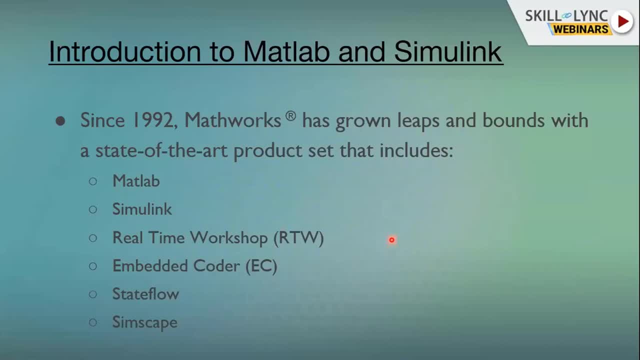 I'm not going to go over any embedded coder element today. They have Stateflow, which is another component of MATLAB, And then Simscape. They have acquired some of these companies. Simscape has tools or block sets to support. When I say block set, it's basically a Simulink-based block set. 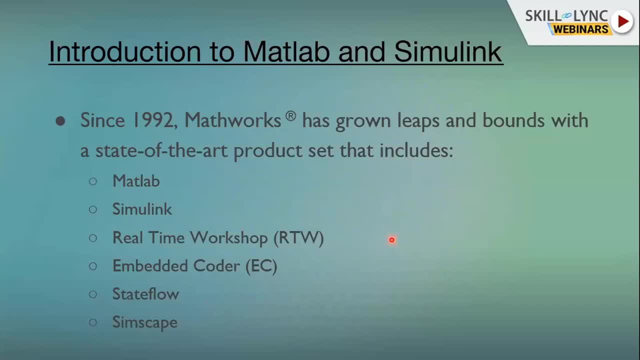 So the Simscape product was originally developed as a competitive product for AMSim with a lot of support for hydraulics modeling And the power systems. also they saw an opportunity to make the power system design as part of Simscape And in addition MATLAB. like I said, they also have block sets. 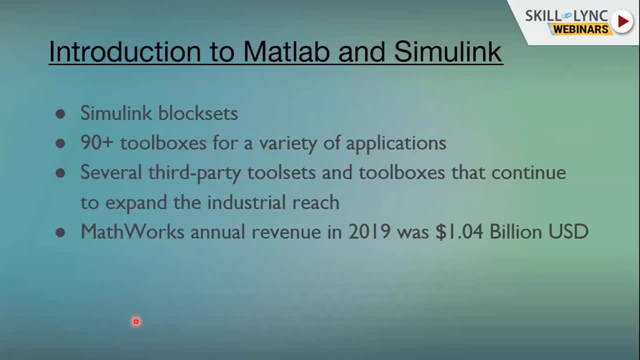 Today they have aerospace block set and Simscape block set, et cetera. So right now, though, they started in 1982 timeframe with 90 plus tool. I mean two toolboxes, But today they have grown to 90 plus toolboxes for a variety of applications. 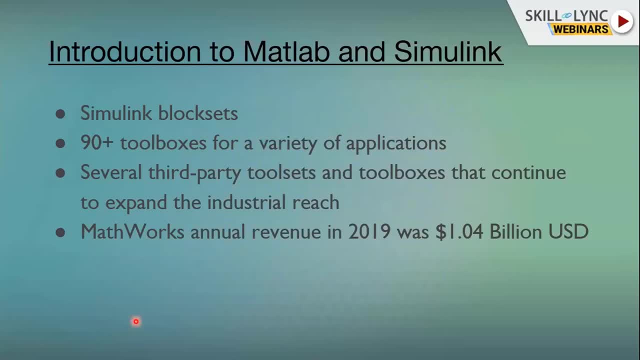 They have machine language. you know tools for machine language: signal processing, image processing, you name it- And they continuously they grow. They continue to grow, teaming up with academia. Anytime there is a new technology out there, they'll try to build a tool. 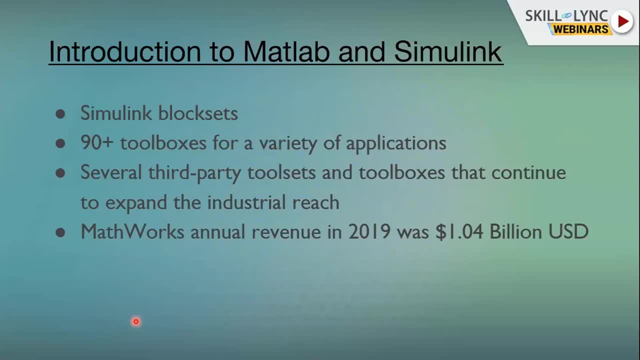 Yeah, They'll try to build a tool set to help the students and engineers, researchers Also. the MATLAB Simulink platform lends itself to the third-party tool set development. So if somebody is trying to develop a cutting edge solution, they could use MATLAB Simulink as the platform and then develop their tools and market them. 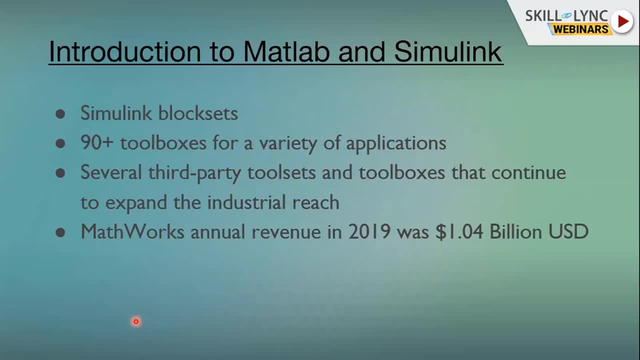 independently, But the requirement would be that you have a used MATLAB and Simulink environment to use their product. Just to give you you know what is the market value of MathWorks today, I mean in 2019,. I have data. 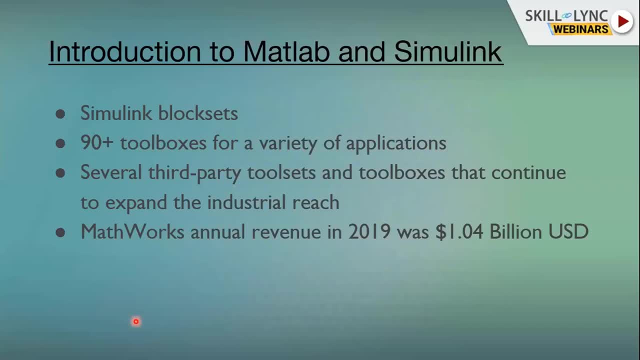 In 2019, it was valued at 1.04 billion US dollars And I used to work for MathWorks. you know way back when, around 2009 frame, I briefly worked for MathWorks And at the time it was valued at 500 million- half a billion. 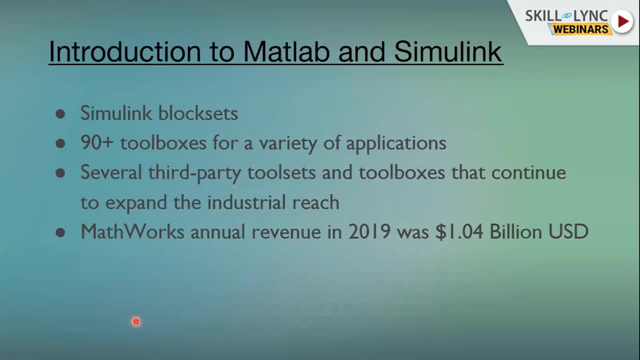 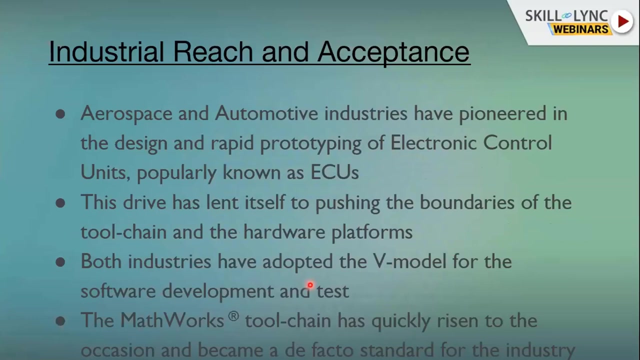 So in the last 10, 12 years timeframe, they have doubled themselves. It is still a privately held company and that's significant. Yeah, And I'm just going to go to my presentation for the second slide so that you can see that it's being made available. 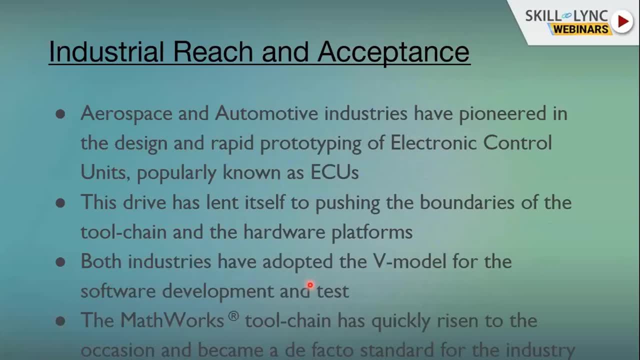 So if you just click the link, I'll show you how I can show you how MathWorks works. So this is just the introduction of our platform. This is just a demo of what we have, what we have developed. Now we have just covered how MATLAB and Simulink have evolved. 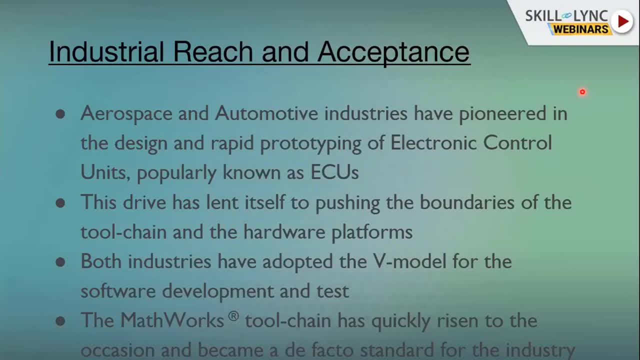 I'm sure other products have evolved, But none of the other products really got to the same level as MATLAB in terms of industrial reach and acceptance. I mean, initially, the other space and automotive industries have pioneered in the design process. So I mean, this is just a demo and I'm just going to go through it now. 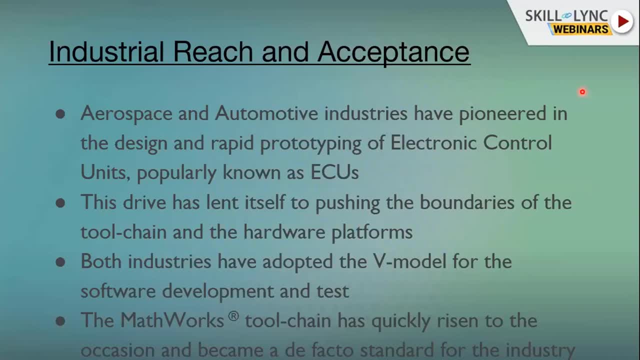 design and rapid prototyping of electronic control units, what we call them ECUs. So those are the two industries. really, Aerospace industry had a lot of money and they were trying to advance their technologies and bring them to the market as quickly as possible. 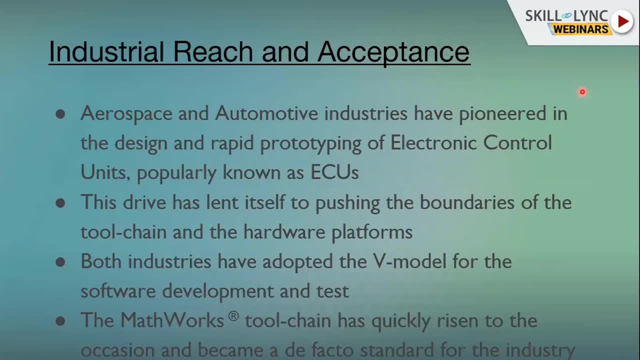 They were initially going from mechanical links to fly-by-wire technologies, Automotive. the fly-by-wire is essentially it's communication, how individual elements, individual components, subsystems of an aircraft communicate. There was a buzz standard called A-ring buzz standard. They communicate on a redundant bus. 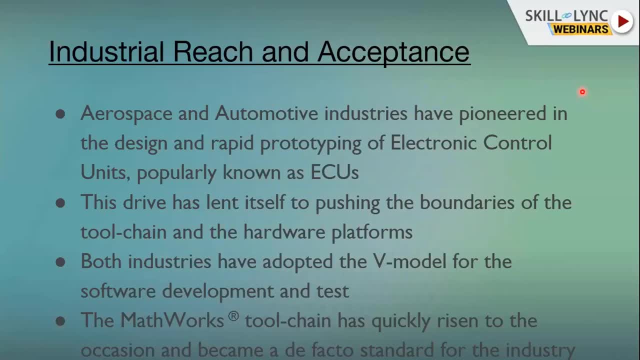 Similarly, automotive industry did the same thing. They have CAN bus architecture, They have flex-ray architecture, They have 이것hip architecture, They have electromotive architecture architecture. Again, we can really draw parallels between automotive and aerospace industries. So 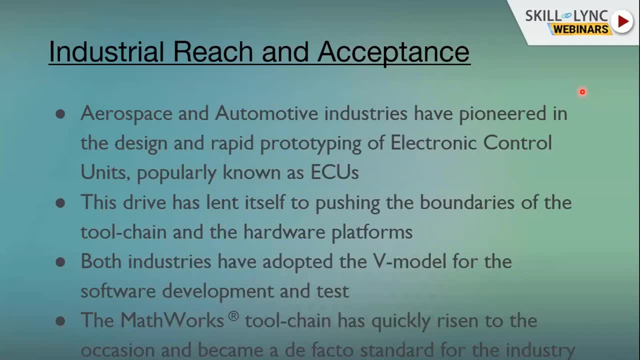 aerospace industry was the brainchild of the innovation and automotive industries, in a way tried piggybacking on that technology that's available to them. So, as these industries were growing leaps and bounds with incorporating ICs, So that itself has given the push to the 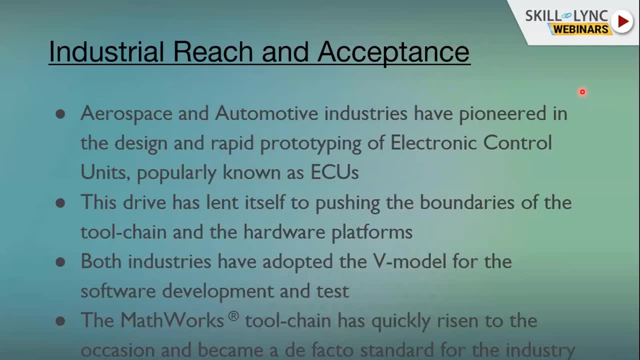 tool chain, For example MATLAB and Simulink, and others might have done the same. They started pushing their boundaries. See what else can be done, What else they can do to help these two industries design and deliver quickly with smaller turnaround times. So the third bullet talks about 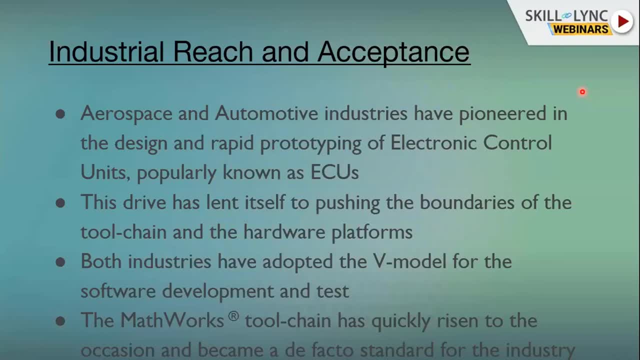 a software development methodology that was evolved from experience and tools available to them, so on and so forth. So, aerospace industry: I have a slide for you. I'll try to give you a little more detail there. But the V model- there are a couple of. 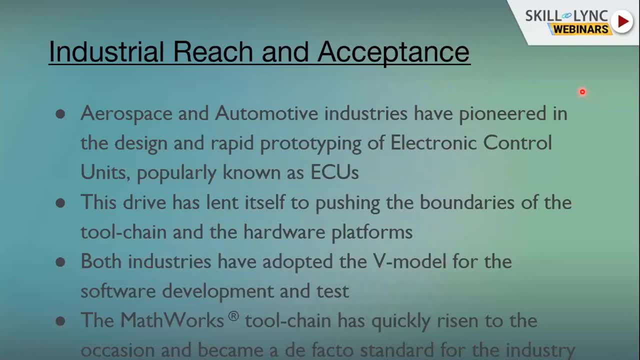 precursors to the V model, There was a software development. I mean, the reason why we talk about software development methodology is because now we have ECUs and you have to install a piece of code and test the hardware in the loop before you deliver the product. 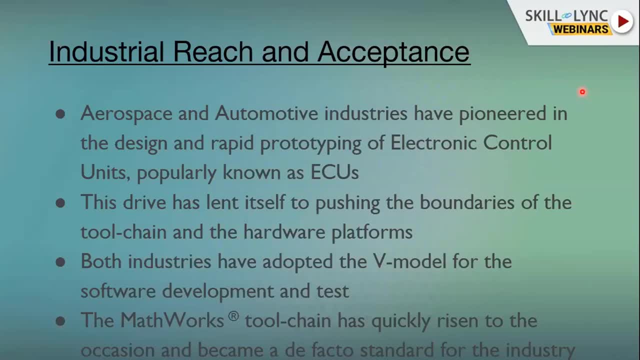 So they needed a software design methodology, so to speak. So the aerospace industry had always used Waterfall. I'm sure aerospace and the software industry have a lot of things in common. The Waterfall had its own drawbacks, So they started adopting game spiral. 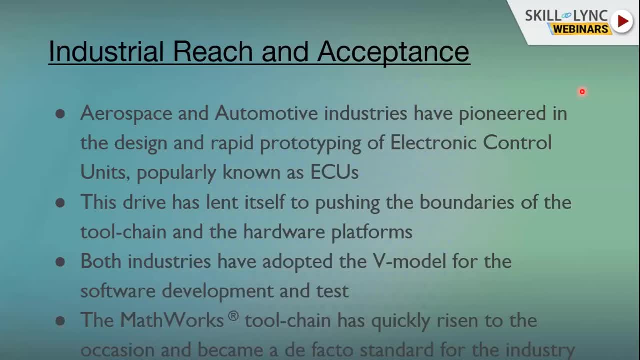 software development model. Now the way the spiral essentially identifies individual subsystems and the interfaces you know, or they try to solidify the interface with experience and what the new innovation might call for. Once the interface ICD, what we typically call it interface control document. once 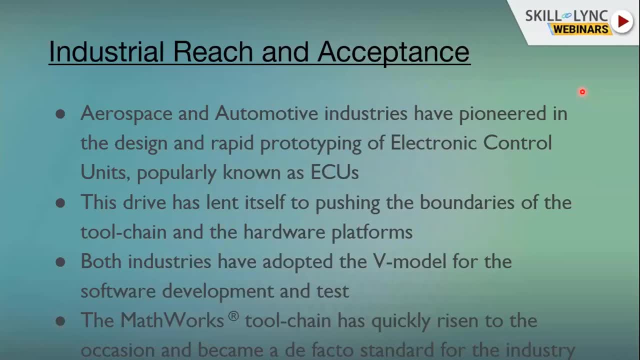 somebody had fleshed out the interfaces, then one could put more meat in the individual subsystems. That's where the spiral, as it was unwinding, are going from the innermost layer to the outermost layer. The fidelity of the models were going higher and higher without changing the interface. 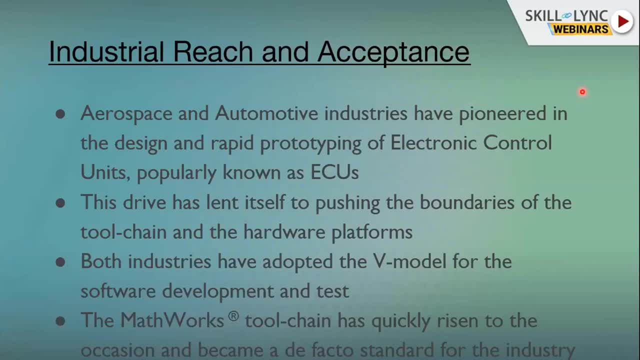 at which point you just go through a series of releases You know, at different stages of the product development. I'm sure some of you know how a product is designed and developed and tested. So you have somebody you know scribbles on a piece of paper and take it through a 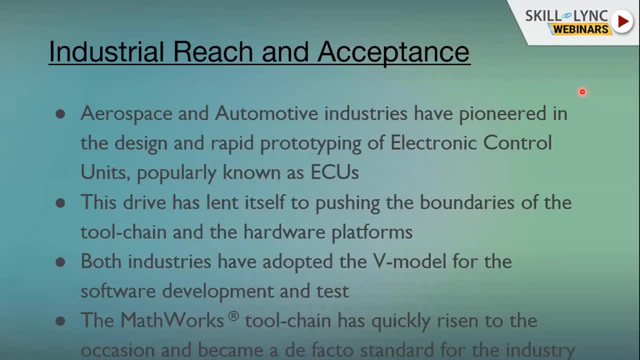 proof of concept stage and then you prototype it and kind of verify validity. You know, you make sure that The technology supports it and it's cost-effective and it's profitable. Ultimately, any product will have to be profitable. It should, you know, generate revenue for the company to sustain and make more products. 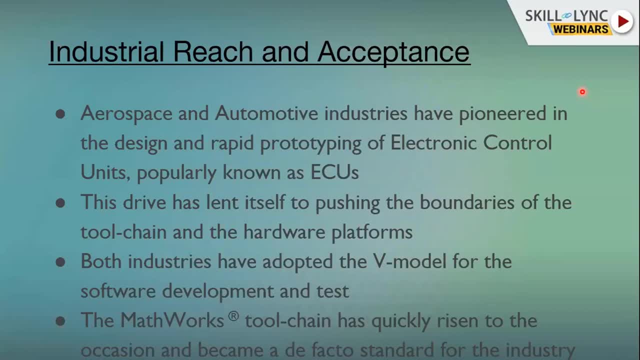 So ultimately, you know the waterfall spiral- all those have culminated in the V model. So, as of today, the V model has been practiced widely by, You know, aerospace and automotive industries. So what MathWorks realized was, again, MathWorks was trying to grow leaps and bounds, as always. 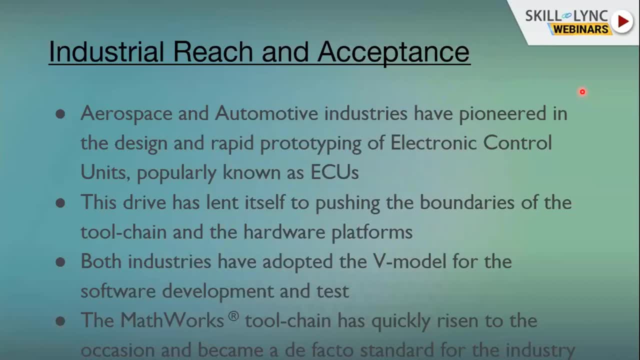 And it has seen the opportunity and they started acquiring a few companies here and there. Speedgoat is one such company. I forgot where Speedgoat is from. It is a- It's a Swiss company, if I'm not mistaken. you know- to help them with real-time support. 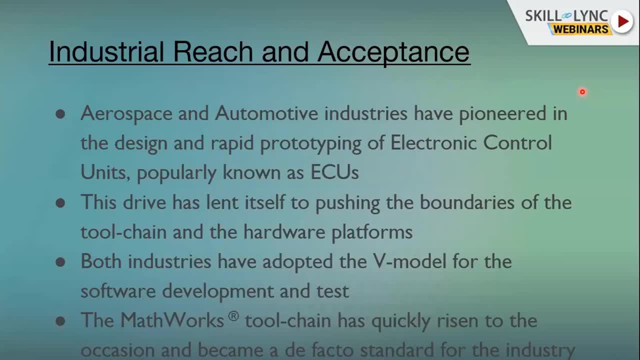 You know MATLAB Simulink. they generate real-time code and it can be ported to the Speedgoat hardware based on your 486, which is our standard PC platforms. We call them the X486 models. You could port and quickly test them. 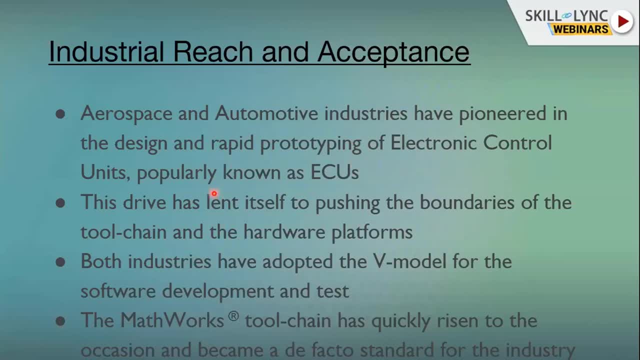 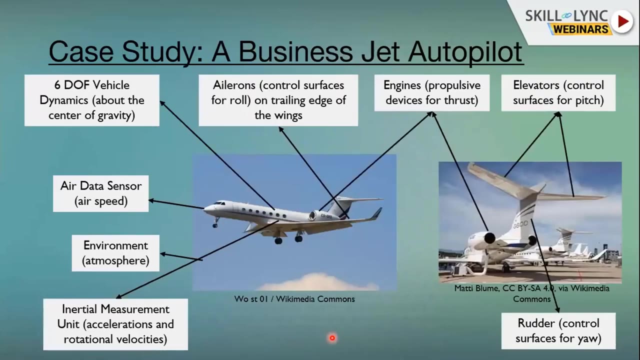 Test the code. So that's the industrial reach and acceptance. So once the MATLAB MathWorks toolchain has become industry standard it was much easier for the industry to take it and run with it. So that kind of covers the history and background of various toolchains and where MATLAB and 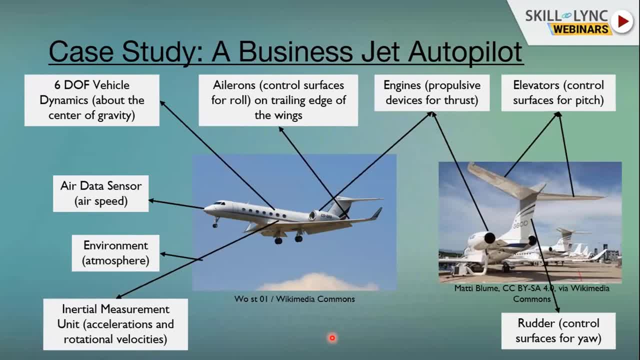 Simulink are positioned. So I'm going to go over in this slide. you know how one would go about designing an autopilot For a business jet. there's no reason why I picked business jet. It could be just any aircraft. 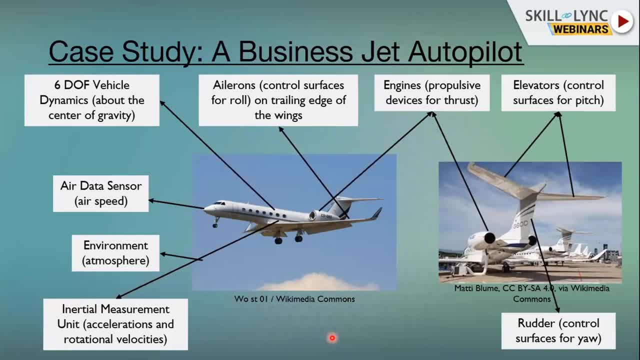 Maybe because I briefly worked for Gulfstream, which is an aerospace company that makes business jets, So I was kind of excited to include that as an example. So an aircraft, I mean, if you think about an aircraft, I mean I picked the aircraft. 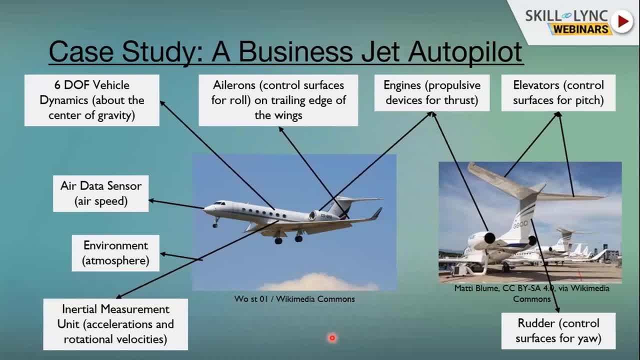 again to show different complexities. you know it's more than complexity. It's highly involved. To come up with a mathematical model for design purposes is involved because it has six degrees of freedom. So I'll go from the left corner and I'll just quickly go over each component of an aircraft. 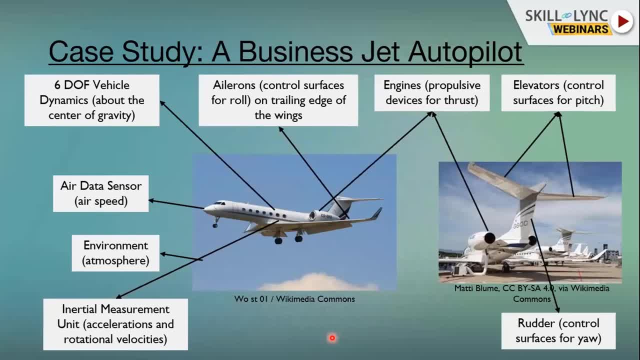 So, as we all know, the aircrafts operate in an atmosphere which is, you know, which is full of air, and air is a fluid, provides the aerodynamics forces, environment needed for the aircraft to fly. The aircraft is equipped with the sensors and actuators. 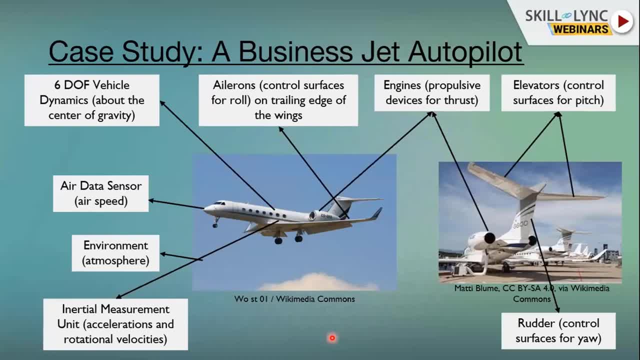 So let's talk about sensors. I mean, there is, we have underlying dynamics. you know, aircraft by itself is a rigid mass And when a rigid mass is subjected to a rigid body, when a rigid body is subjected to forces. so you have you know. 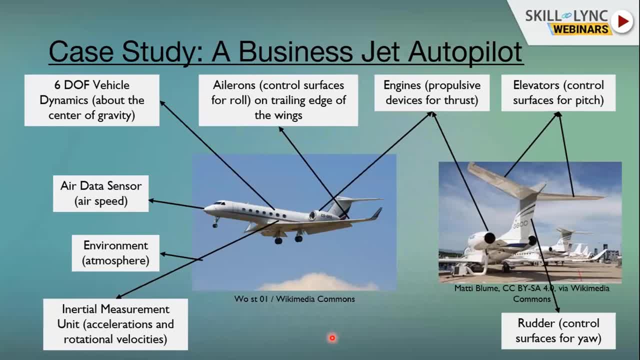 when you apply forces to the rigid body, you start seeing its motion. basically, So inherently, an aircraft is treated to have six degrees of freedom, The reason being so it has. I mean in a three-dimensional space. we normally represent three-dimensional space with the x, y and z axis. 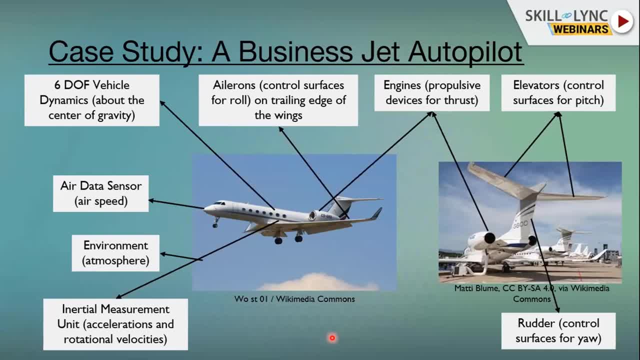 which means there are three degrees of freedom there. So the aircraft can move translationally along x, y and z-axis, or it can also rotate by virtue of its being airborne. It can rotate about x-axis, y-axis and z-axis. So there are three translational degrees of freedom and three rotational degrees. 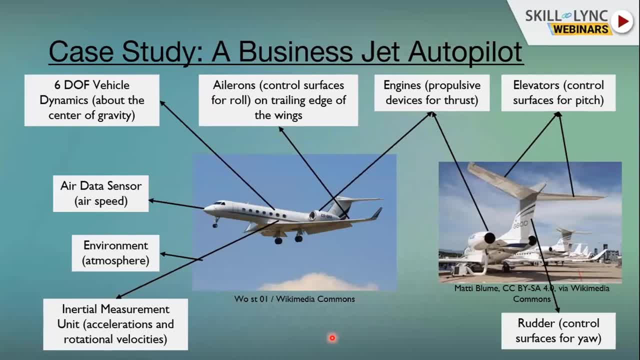 of freedom. that makes it six, And the equations of motion are generic. What makes the equations different from aircraft to aircraft is basically the parameters: The size, what control surfaces you have. what are the sizes of the control surfaces, what propulsive device you have. 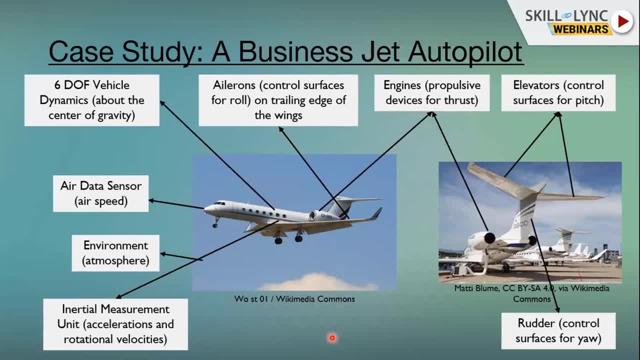 So the aircrafts need engines to generate forward thrust. Here I'm showing a two-engine configuration. You also might have seen a single-engine configuration mounted on the tail. So there are all kinds of configurations and one needs to build a model before a design. 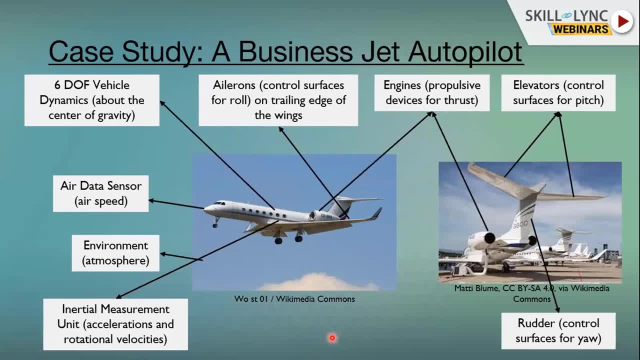 can be thought about. So, going back to the details of the slide, so we talked about the aircraft, the rigid body, dynamics, which has six degrees of freedom, And then the aircraft is equipped with all kinds of sensors. At a minimum, it needs to have an. 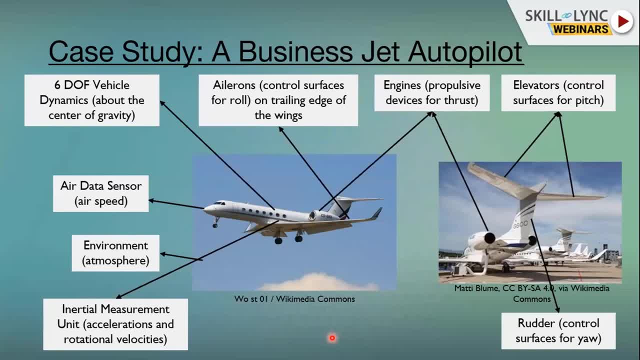 inertial measurement unit that has accelerometers and gyros to measure accelerations and rotational body velocities. It needs an air data sensor to determine the speed of its own self. It also has an altimeter, which I'm not showing here. The altimeter determines or measures the 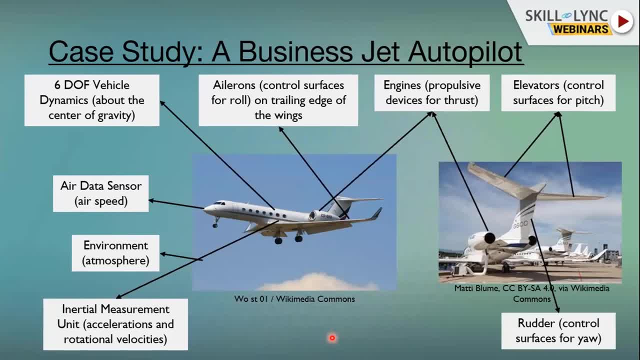 altitude, how far away you are from the ground. That's another sensor. And now, speaking of controls, so the aircraft is equipped with all kinds of control surfaces. You have ailerons to help the aircraft roll. When you deflect the ailerons, the aircraft.